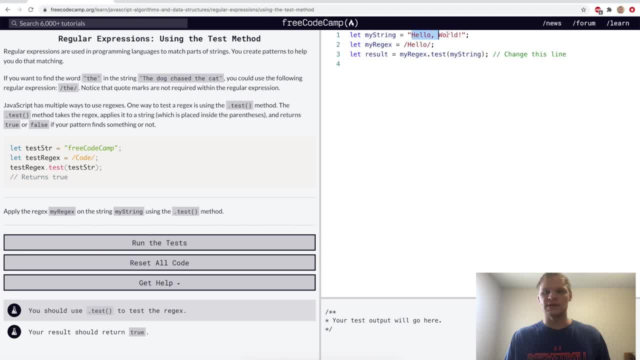 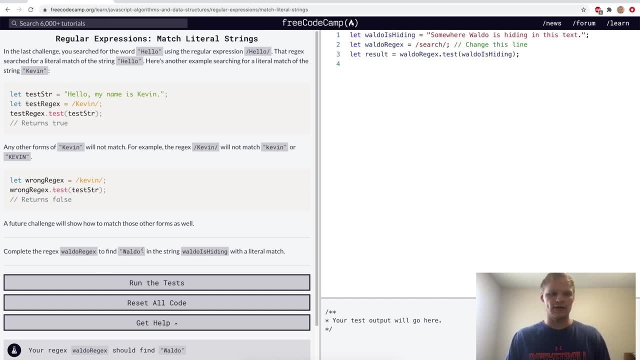 string And it'll return true if hello is found inside the string, which it is. so it should be true. And let's try that. Yep match literal strings Here. we want to find Waldo in this string, So instead of search, here we can. 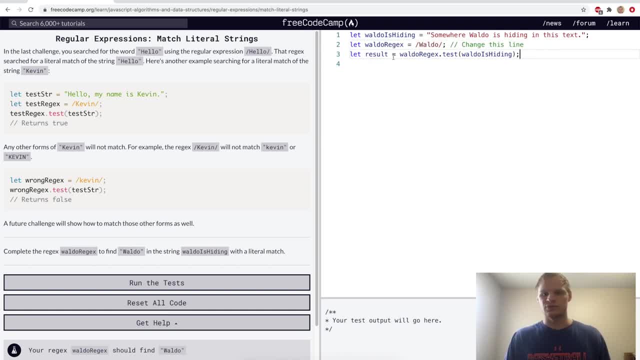 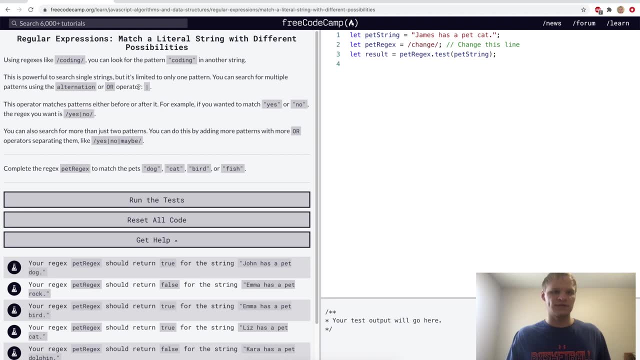 put in Waldo And now result will turn true. So let's try that Yep match a literal string with different possibilities. We can do this with this pipe which stands for or So in this case we want to do dog or cat or bird. So dog or cat or bird, or even fish. And since cat is in the string, 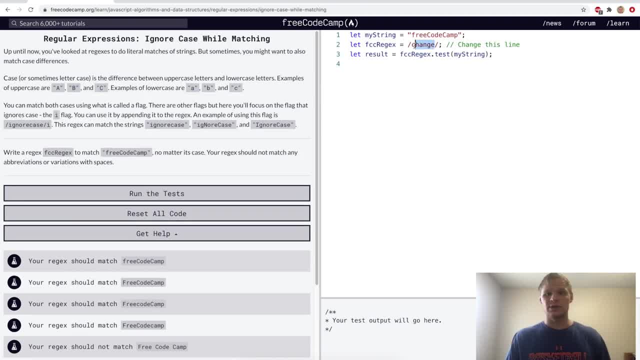 result should be true: Ignore case while matching. Here we can put an i at the end of the backslashes and that will mean it's case insensitive. So here we'll do free case CodeCamp And it will still be true even though it doesn't match the case. 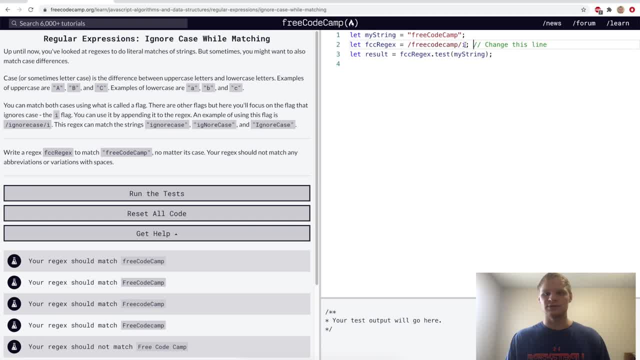 correctly, because we put an i at the end And there's other special characters that you can put back here, like g and some others. But i is used quite a bit because sometimes we just need to match a string of characters and not worry about case. So let's try that. Yep extract. 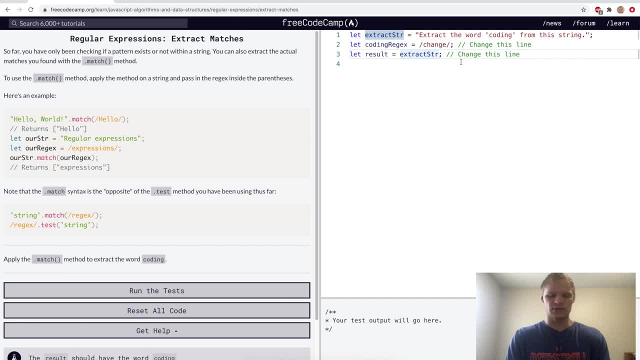 matches. Here we want to do our exact string dot match and then we can pass in our coding rejects into it. It's the opposite, as the test method like this explains, And we want to find the word coding. So there we find the word coding and then we match it. 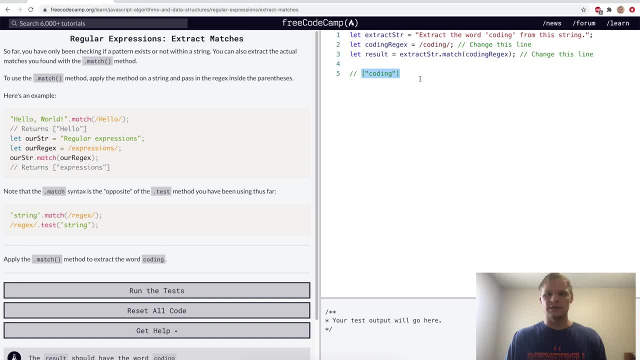 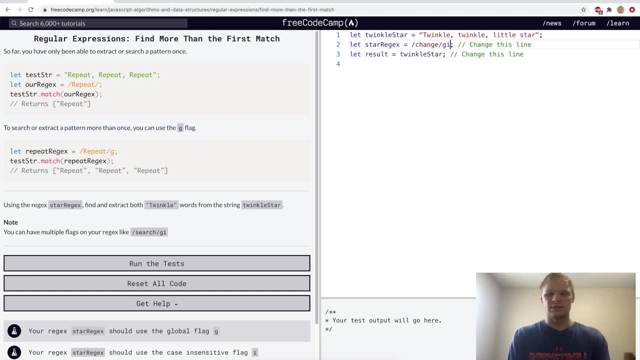 And then the result becomes an array of that word. Let's try that Yep find more than the first match. This is done with the g flag, So we can have g and i back here, which stands for global and insensitive to case, And we want to find twinkle. So now it'll find this one and it'll. 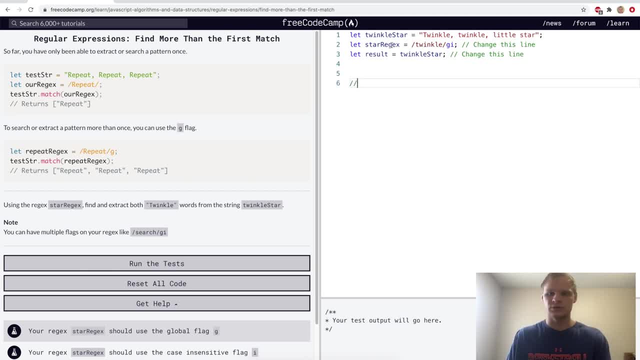 find this one and put it in an array like this: Oh, actually we want to match as well, Match star, and let's console log the result just to show. So yeah, there's the result. Twinkle and twinkle, Let's try it. Yep, match anything with the wildcard period Here we want to match run. 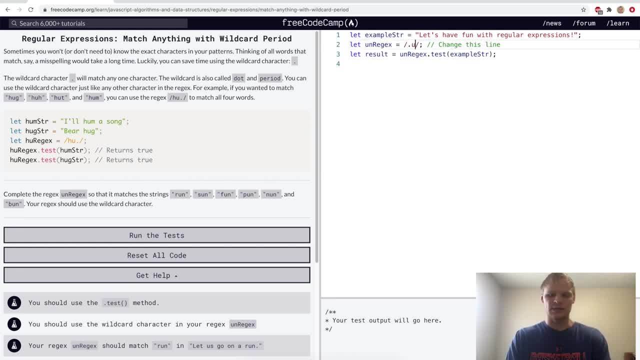 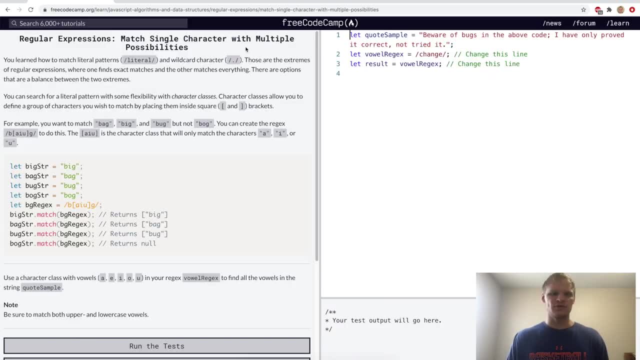 sun fun pun none and bun. And the way we can do that is by doing dot un And that should work for this test. So it'll find fun and result should be true: Yep. match single characters with multiple possibilities. This is done by using brackets. So first of all we want to match. 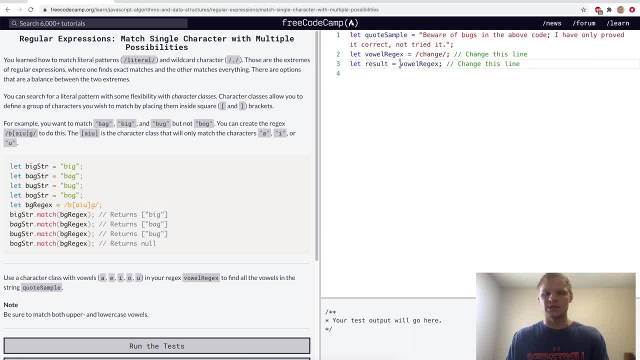 our rejects. But of course we want to do quote, sample, dot, match, Match, the vowel checks And then change this so that it finds all the vowels A, E, I or U. And then we also want it to be global so that it finds all of them, And also case insensitive. And I think 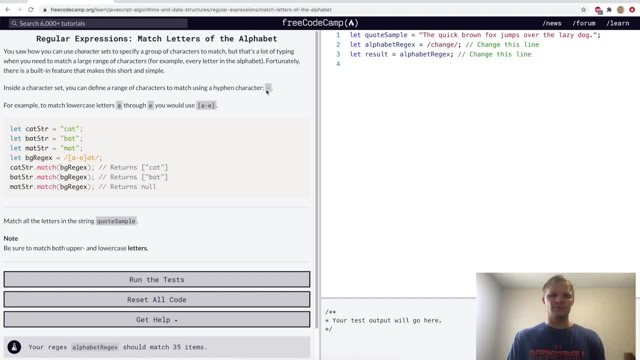 that should work. Let's try it. Yep, match letters of the alphabet. Here we can select a bunch of letters by doing A through another letter And it's in alphabetical order. So we can do A through Z and it'll match all the characters. It'll match all the letters at. 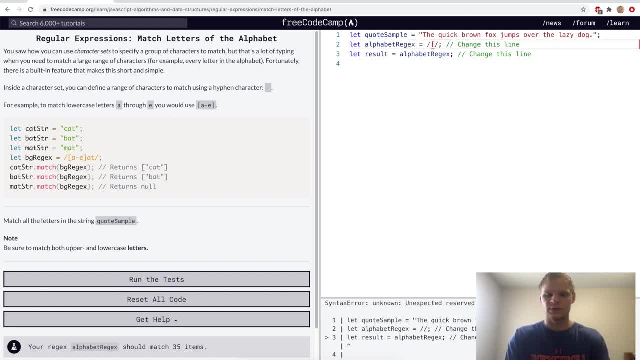 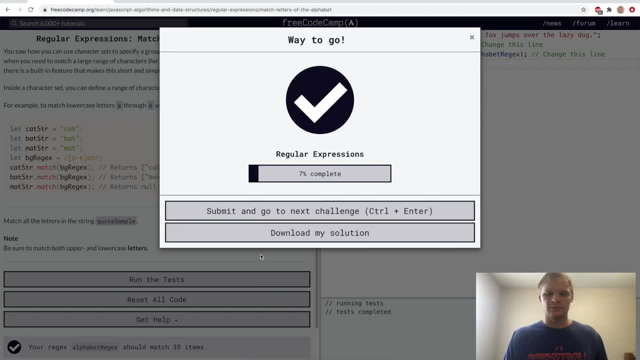 least. So here we want to match all of these. So we'll go A through Z, Case, insensitive and global, And then we'll do quote sample, dot match And we'll match it with this rejects And let's try that, Yep, match numbers and letters of the alphabet. We can also do this thing with numbers. 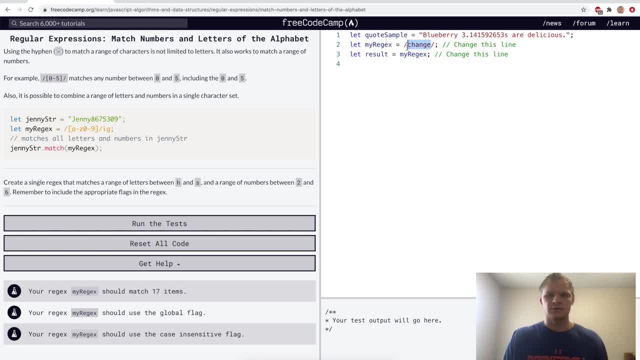 as well. So the same as we do A through Z, we can do 0 through 9.. So for the challenge we want H through S and 2 through 6.. And then case insensitive and global as well. And then do quote sample: dot match again, Match it with the rejects and try it: Yep match single characters. 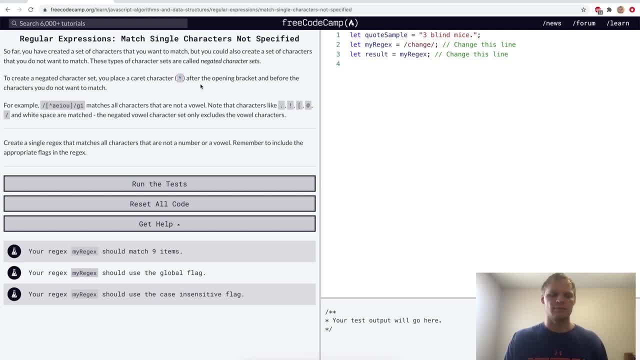 not specified Here we can use this carrot operator to say anything that's not this. So for the challenge, we want to have a rejects that matches all characters that are not a number or a vowel. So here we'll change this to being not So, not with the carrot, And then 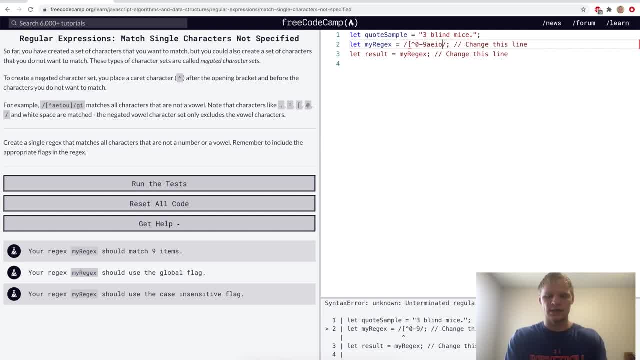 a number, So 0 through 9, or a vowel, which is A, E, I or U, And then we'll set the global flag and the case insensitive flag And then we'll do quote sample dot match on my rejects and run it. 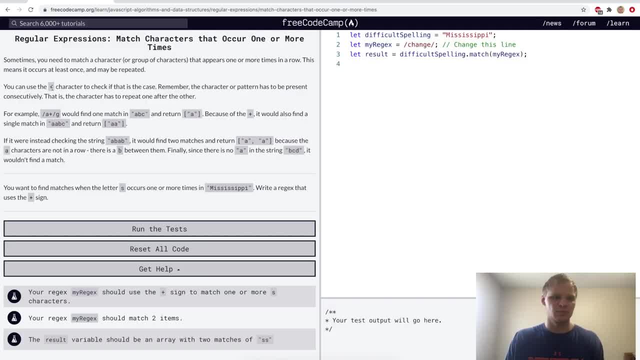 Yep match characters that occur one or more times. This is done with the plus character For the challenge. we want to find where S occurs More than once. So here we'll do S plus and then we'll set it as global, And we also don't want it. 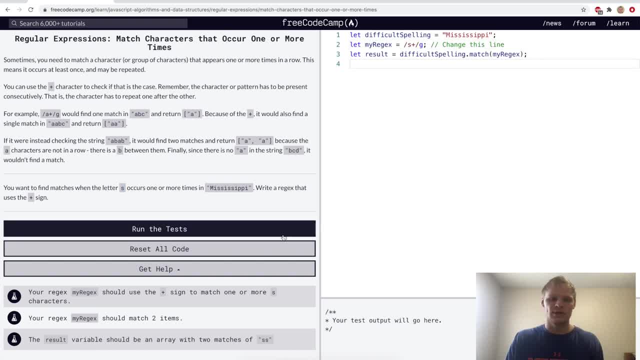 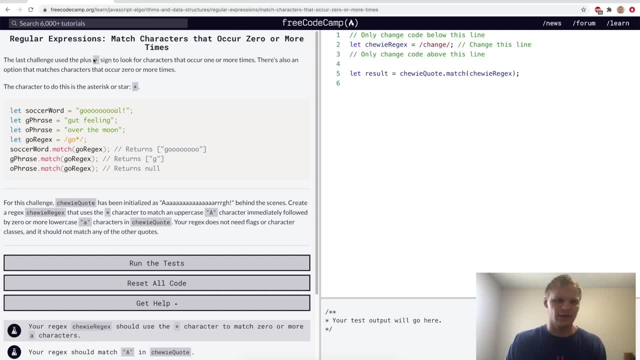 to be insensitive because we want lowercase S's And then try that out: Yep, match characters that occur zero or more times. This is done with the star character. It's exactly like the plus sign, except it does zero more times instead of one or more times. And for the challenge we want to have. 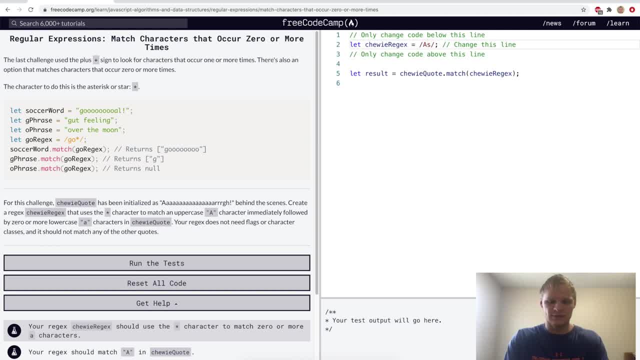 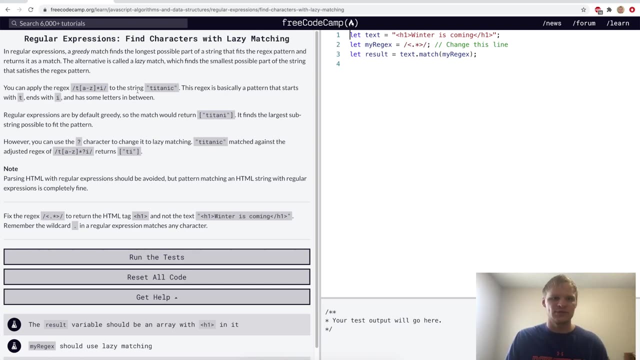 this be uppercase A and then lowercase a, followed by followed by an asterisk or star, And that will all the way up to the last a. So let's try that Yep find characters with lazy matching. So by default, regular expressions are greedy, which means they try and find the longest possible. 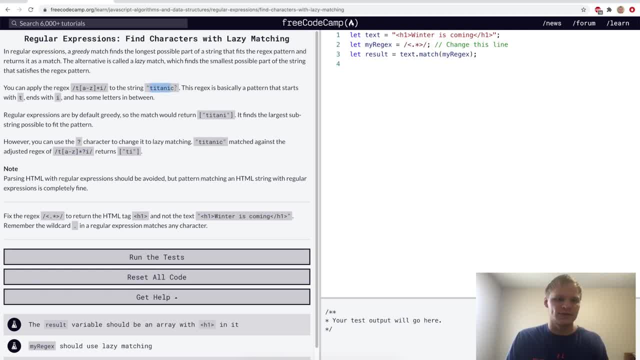 substring that matches. So the example they give is with Titanic. They want to find T A through Z and I And it'll find Titanic instead of just tie, even though tie matches as well. But the way that we turn off the greediness of regular expressions is by putting a question mark character in inside. 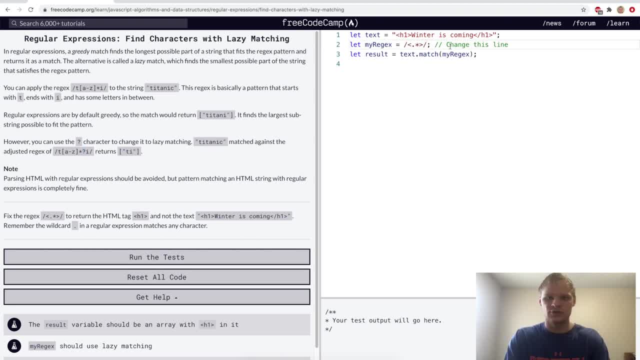 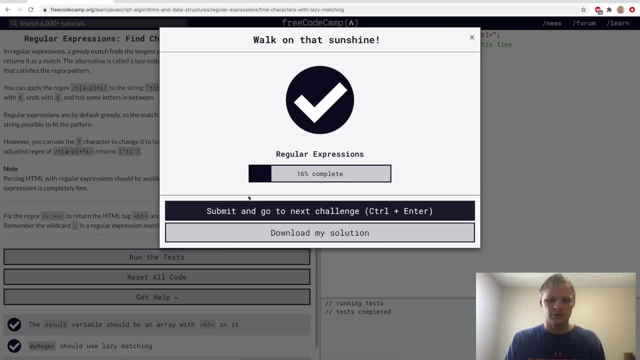 the regular expression, And that will make it not greedy anymore. So for the challenge, we would just want to add a question mark here, And that way it'll just grab the h1 here instead of the whole thing. So let's try that Yep find one or more criminals in a hunt. Here's a little. 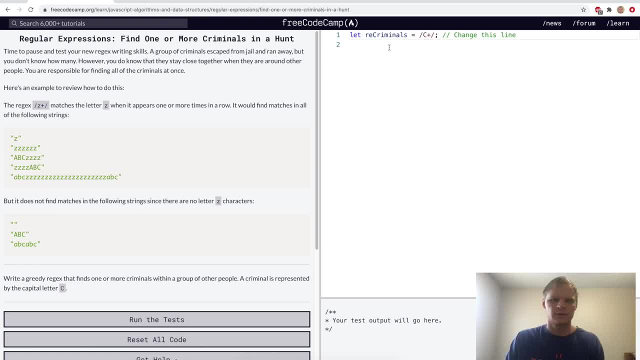 challenge by FreeCodeCamp And I'll complete it and then show you after. Okay, I think all we needed was a capital C plus, And it'll find one or more criminals within the group of other people, because the criminal is represented by the capital letter C. So let's try this, Yep. 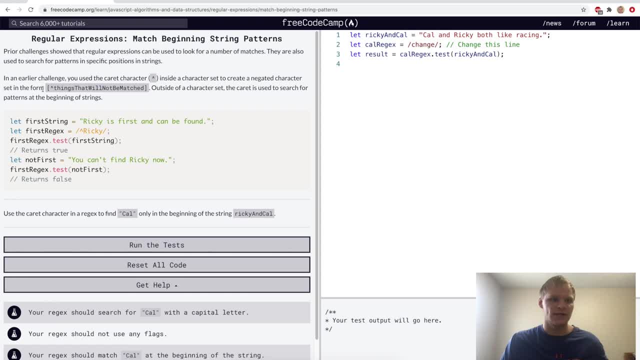 we're going to use the ending string patterns. This is done with the caret. We used caret inside of the brackets before to negate whatever that was, But we can also use it outside of the brackets And that just means that it'll check the start of the string. So here we'll do caret cal And it'll 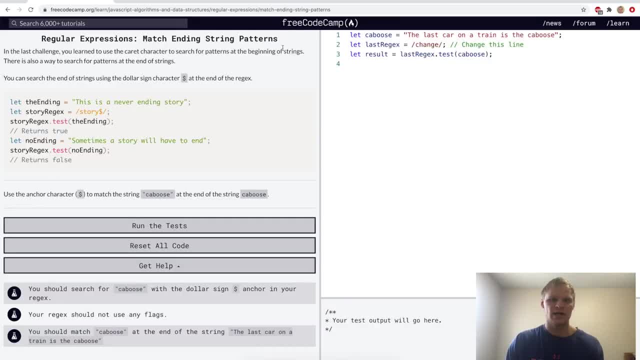 match up with cal here. So let's try that. Yep match ending string patterns. This is done with the dollar sign at the end of a regular expression, So kind of like the caret at the in the other one. Here we want to find Caboose at the end, So we put a dollar sign. 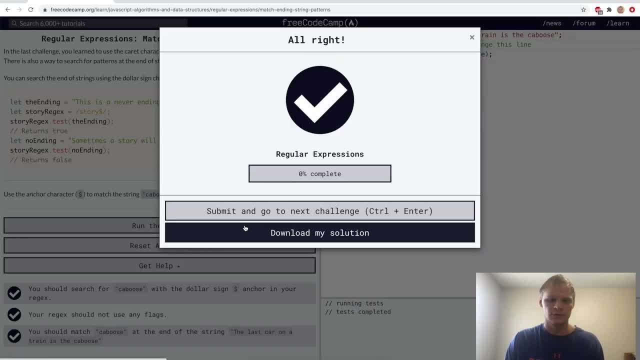 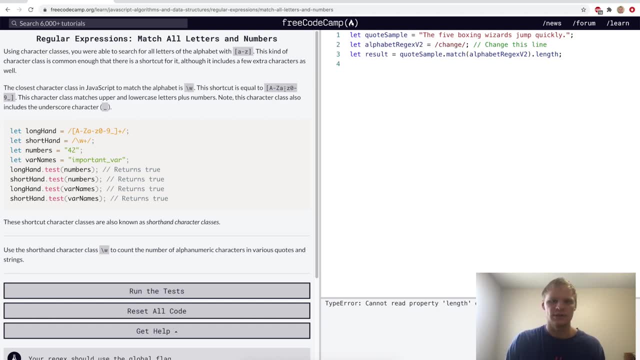 up with this caboose here and return true match all letters and numbers. this is done with the backslash w, it's the shortcut equal to a through z uppercase, a through c lowercase and zero through nine underscore. so here we'll just do backslash w and then we'll go case insensitive. well, actually. 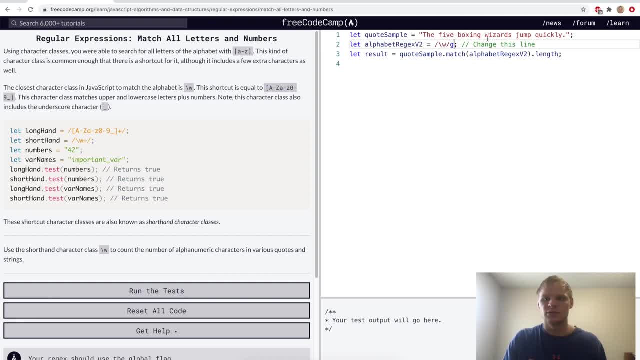 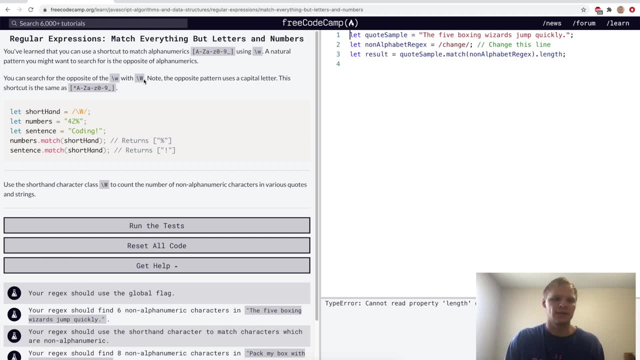 i don't think you have to even do that, but we also want it to be global. so it finds all of them and let's try that yep match everything but letters and numbers. this is done with the capital backslash capital, w, and it's the same thing as not a through z, a through z, zero through nine. 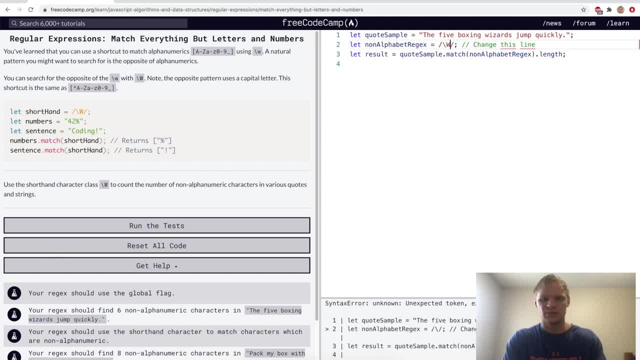 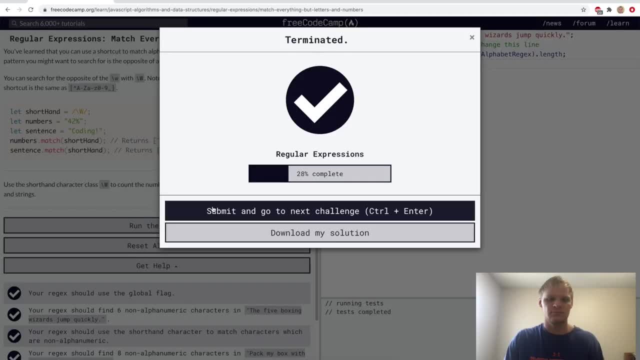 underscore so it changes us to backslash uppercase w and with the g flag find all of them. and i'm guessing it'll only find the dot. but yeah, let's try it. yep, match all numbers. we can do backslash d to match zero through nine. it's just the shorthand way of doing it, so you can just think. 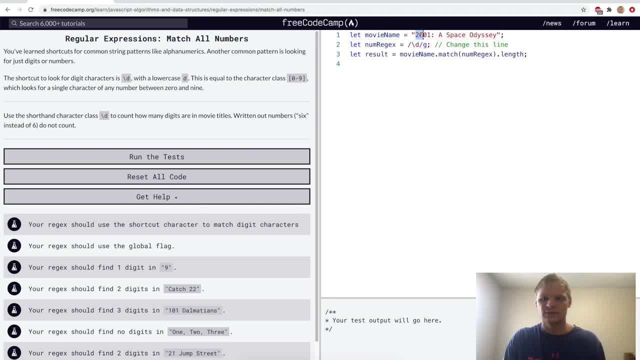 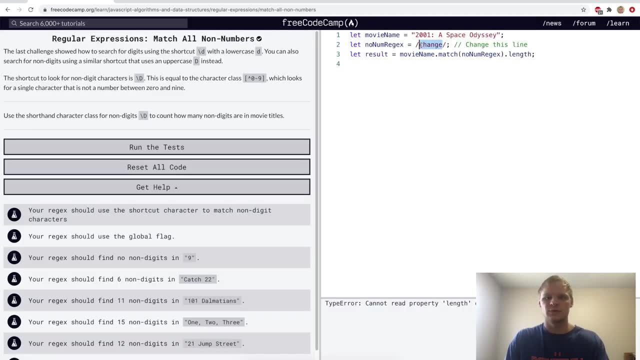 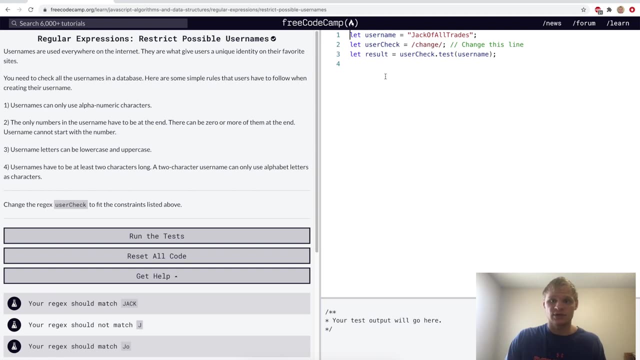 digits, and then we'll set it to be global as well. so it finds two zero, zero one, and let's try that yep match all non-numbers with backslash uppercase d. so here we'll do backslash uppercase d and g flag as well, and try that yep restrict possible usernames for this challenge we want to make. 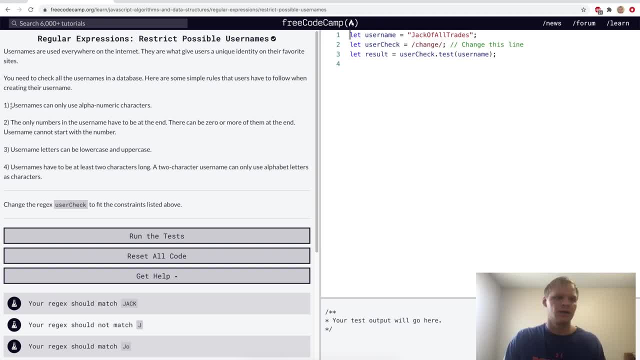 a regular expression that checks if a username is valid. and a username has to fit all four of these criterias. they can only be alphanumeric characters, numbers in the username have to be at the end, they cannot start with the number, they can be lowercase or uppercase and they have to be 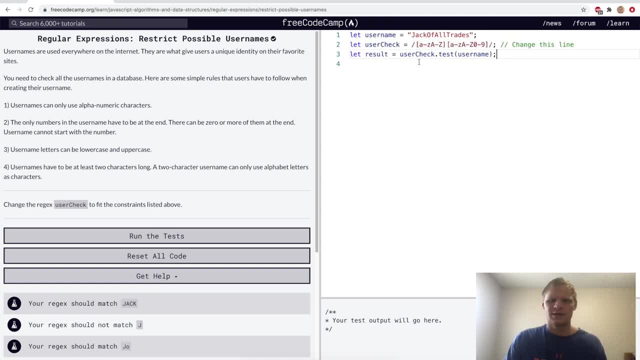 at least two characters long. so i'll see what i can come up with and show you. okay, i think this might work. so it checks a through z, a through z. oh, maybe i'll so. so it makes sure it has a letter at the beginning, and then you can use numbers afterwards, and then it has to be at: 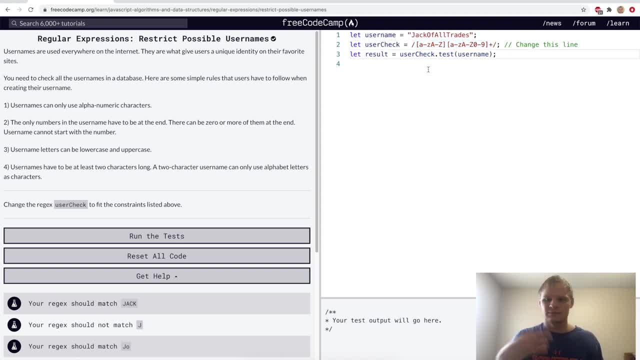 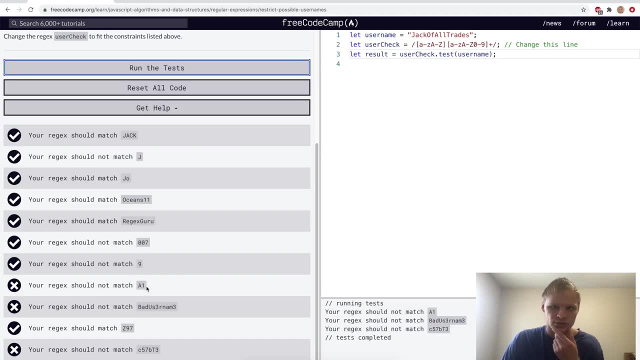 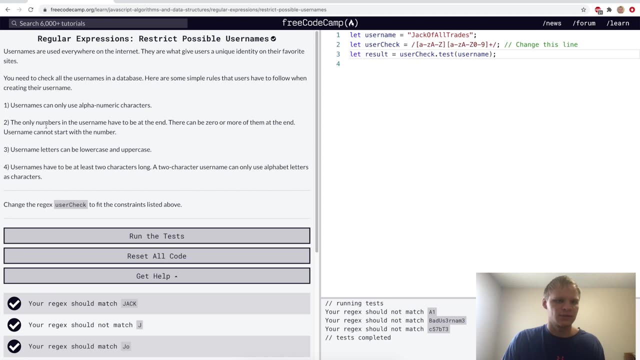 least these two characters long, and then the plus sign to do one or more of these. so let's try. this looks like it doesn't match a1, or it does match a1, but it shouldn't. and it matches this, but it shouldn't. and it matches this and it also should not. i think that's because the only numbers in 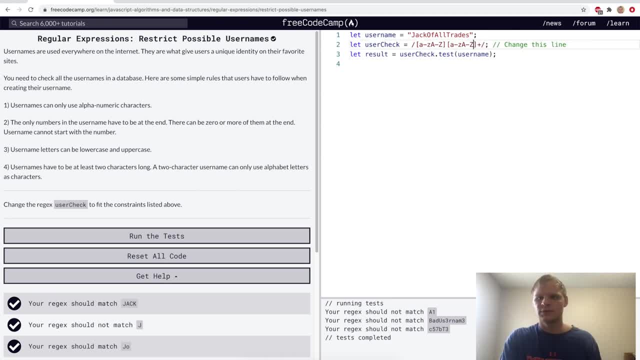 the username have to be at the end. so i'll see what i can come up with and then i'll see what it looks like at the end. so i think first i'll get rid of 0 through 9 here, then maybe i'll put the 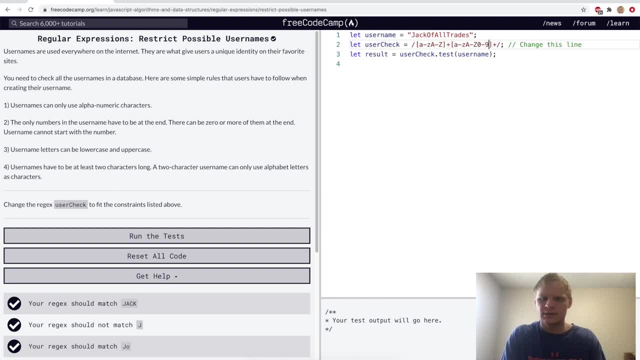 plus in the middle and then do 0 through 9 at the end. so maybe all i had to do is move the plus to the middle. let's try that out. same problem, all right. here i had to use a hint from free code camp, but i'll try and explain what this is doing. so the carrot at the beginning is checking at the. 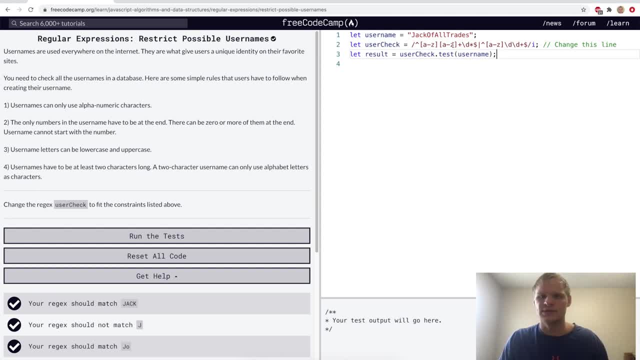 start, that the start matches a through z, a through z, and then we can have as many of those characters as we want after those two, and then we can have digits afterwards and zero or more of those digits, and then we can have as many of those characters as we want after those two, and then we can have: 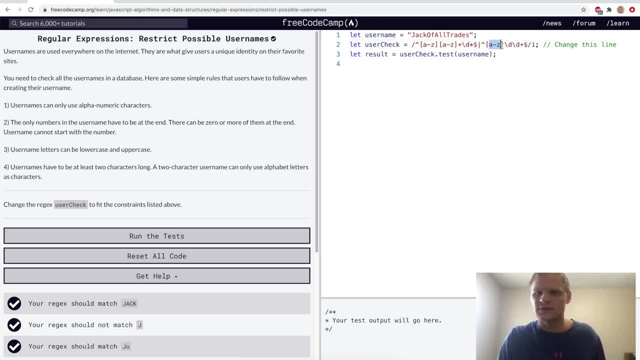 the dollar sign means at the end, or we can do a through z at the start with a digit, as long as there's another digit following at the end, and then it's case insensitive. so this is a through z and uppercase a through z. so yeah, hopefully i explained that decently. let's try it. yep, match. 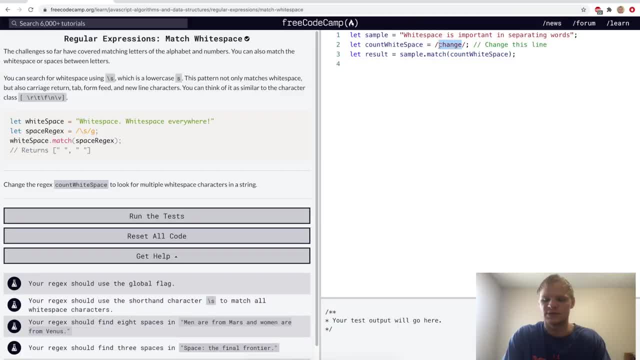 white space. that's done with backslash s. so here we'll change this to backslash s and then we'll check globally. so it'll basically just count the amount of spaces in here, which there is five. so if we did dot length here then it result would be five, but right now it's just an array of five. 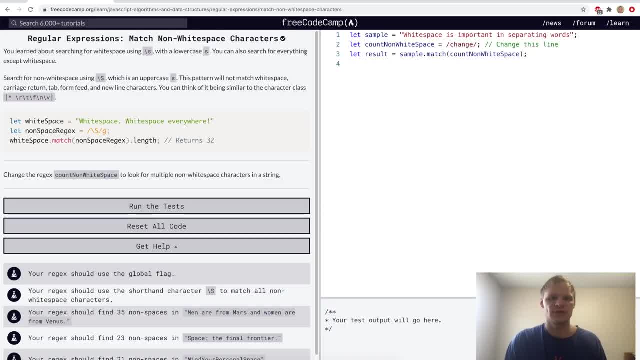 spaces. so let's try that. yep: match non-white space characters. that's done with a backslash uppercase s, so it'll find all these words and not the spaces. let's try that. oh, it needs to be global. now let's try it. yep: specify upper and lower number of matches. that's done with brackets. 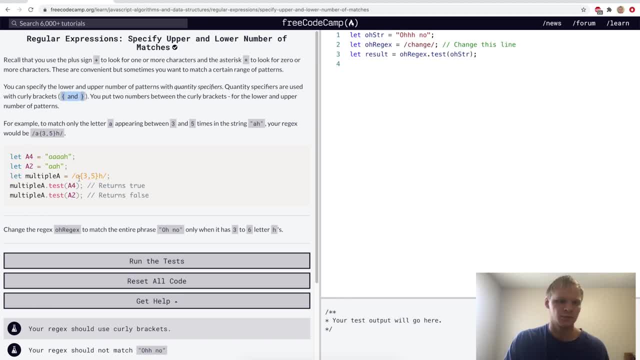 like this example. here there has to be three to five number of a's for it to match. so for the challenge we want to check if there's three to six number of h's. so we'll start with an o and then we'll do h bracket three to six and then we'll go backslash. s for white. 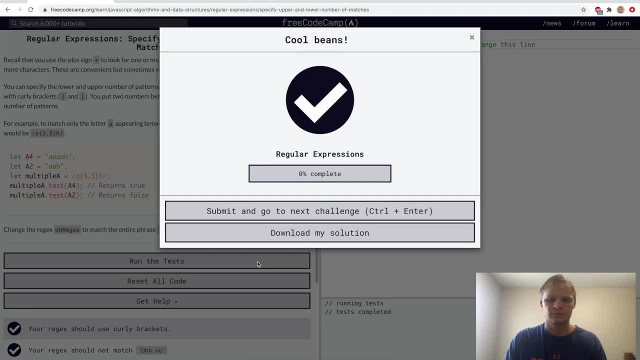 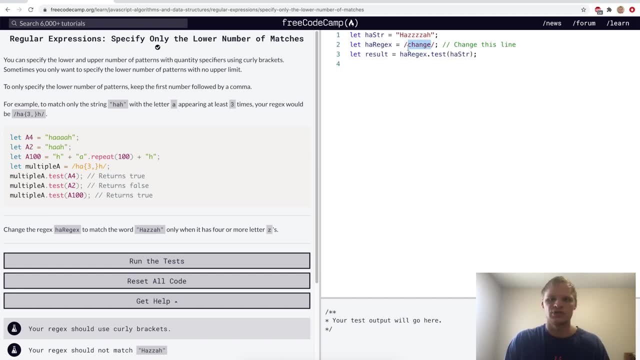 space and then no, and we'll try that out. yep, specify only the lower number of matches. this is done by not even giving a second number to the brackets. so we'll change this to be h, a z and then bracket four or more. so we'll go four comma and then bracket, and then a h at the end, and let's 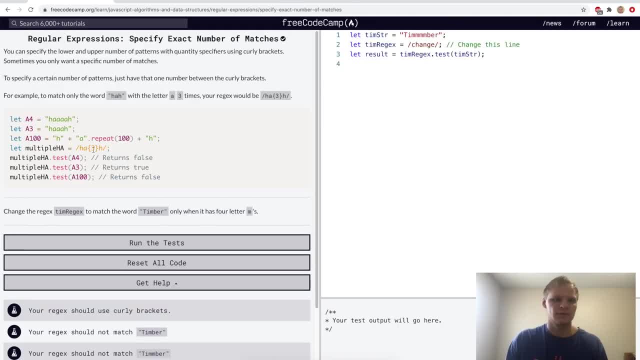 try that out. yep, specify exact number of matches, that's done with just a number in between the brackets. so we'll try that out, and then we'll try that out, and then we'll try that out, and then. so here we want to check if timber has four m's, so we'll go m four of them and then ver. let's try. 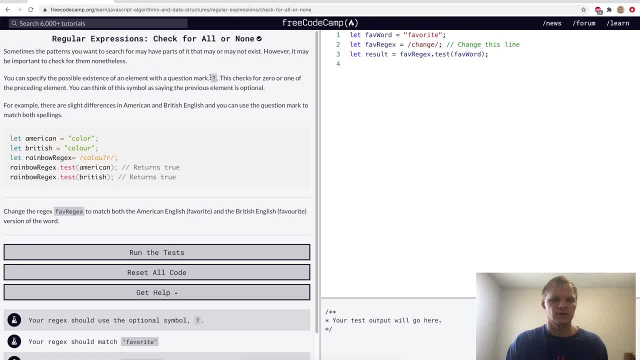 that yep check for all or none. that's done with the question mark after a letter. so here u is questionable if it's in it and it'll match color or color. so u doesn't even have to be in it for it to match. so here we'll change this to be fave for it. and then u is optional after the o, so we'll. 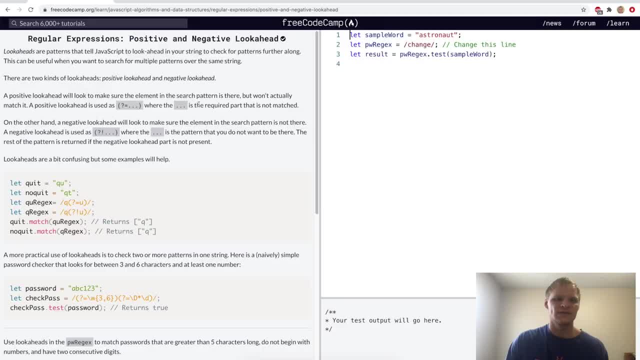 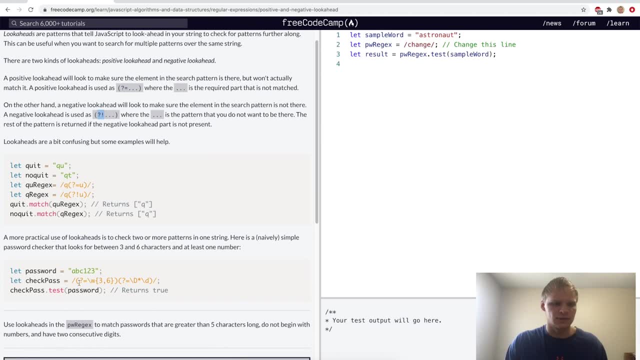 go u question mark and that should work here. yep, positive and negative lookaheads. this is with the question mark exclamation point. a practical use of this would be to check if a password has at least three to six characters of words or of letters, and then three to six characters of. 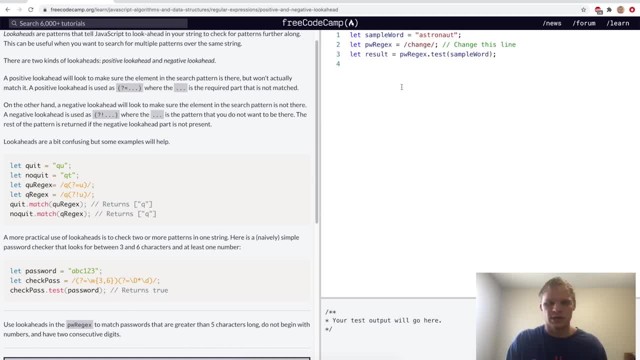 numbers. oh, at least one number actually. so for the challenge, we want to create a rejects that matches passwords that are greater than five characters long, do not begin with numbers and have two consecutive digits. so we'll go with a carrot to check the start and make sure there's. 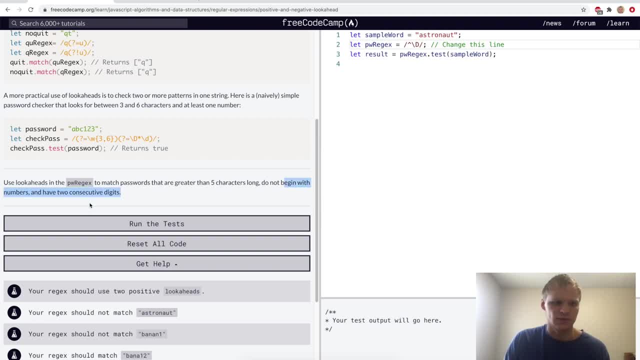 not a digit with capital d. so that checks that it doesn't begin with numbers, and then we'll make sure it's five characters long by doing question mark equals backslash w of five comma. actually we probably don't need a comma there. but then the next part: we're checking if 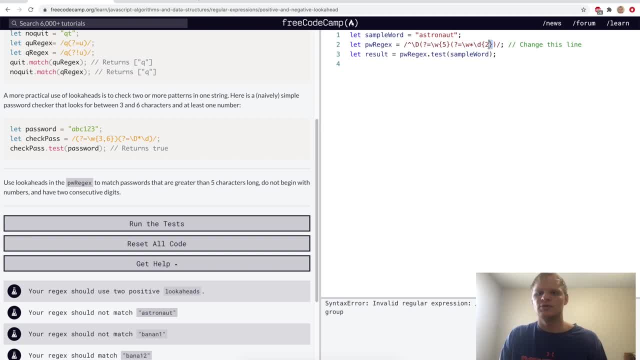 there's any number of characters after that and that there's two consecutive digits inside of the string. so let's just console log some of these quick. make sure there's a parenthesis here as well. so right now it's false because there's no two consecutive digits in here. but as soon as i add, 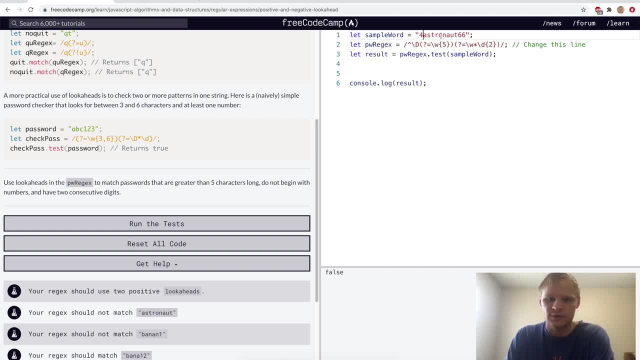 some digits, then it's true. if i put a number at the beginning, then it'll be false. it seems like so. maybe if i have less characters, then it'll be false again. yep, so it has to be five characters long, and let's try this out. yep, check for mixed grouping of characters here. they're checking if 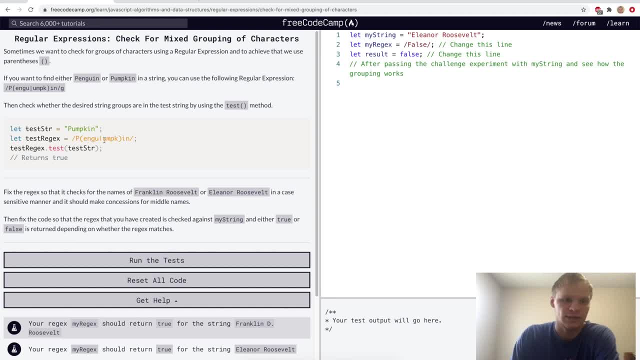 there's penguin or pumpkin by using parentheses and by using the or so for the challenge. we want to check if it's eleanor roosevelt or franklin roosevelt. so we'll go franklin or eleanor and then backslash s for white space and then roosevelt, and then we'll change the result to test that. so 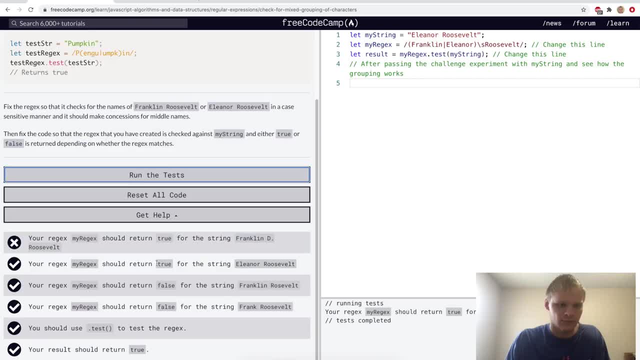 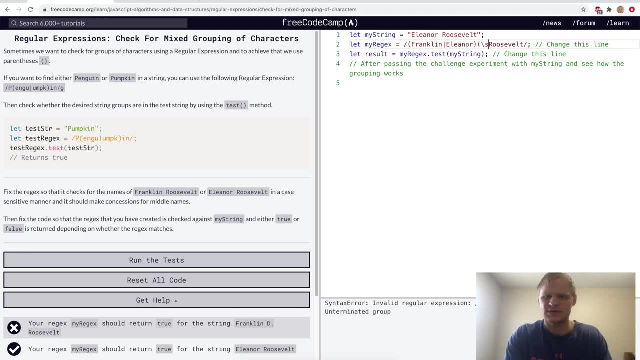 we'll go my rejects that, test my string and let's try that out. oh, it looks like it should match franklin d roosevelt as well. so we'll go backslash. so we'll do another set of parentheses, and then it can be a space, or it can be a d. 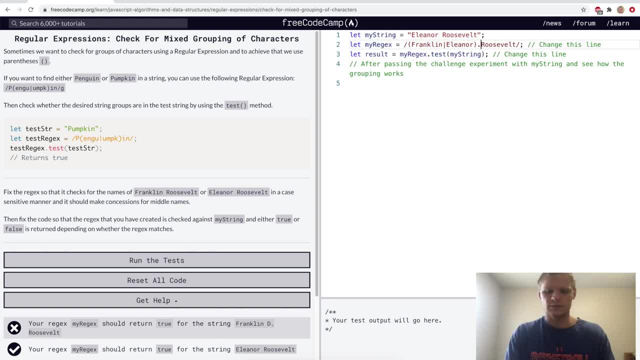 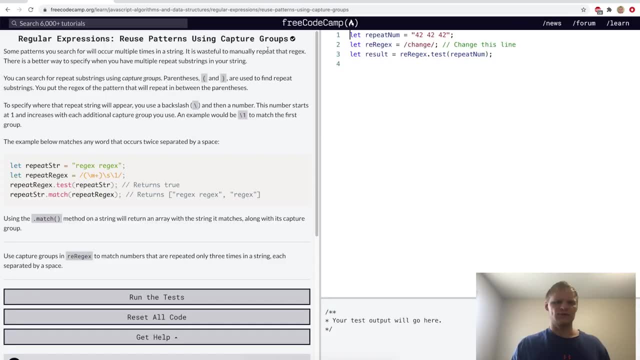 actually for the middle name. we'll do wild card, so dot and then star, so any number of characters for the middle name, and let's try that. yep, there we go. reuse patterns using capture groups. it's done with backslash and then a number. i'm not entirely sure how. this would be super useful, but 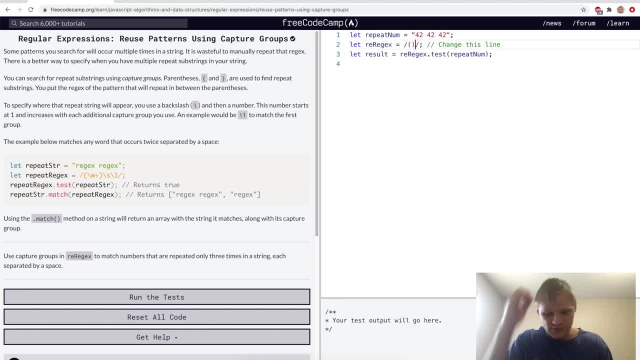 i'll try doing this challenge here. we'll start with parentheses and do a backslash digit with a plus, so it can be any number of digits, and then we'll go backslash s for white space and backslash one to start at the first one. not sure if this will work, but let's try. 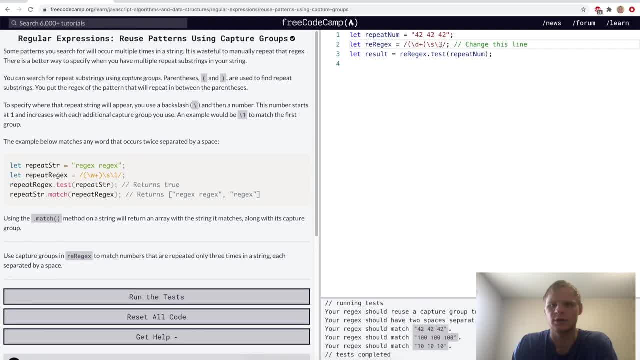 it. nope, maybe if i change it to three, try that. okay, i think i understand the backslash number thing now. so backslash one means this group. so it'll go, it'll check for the digit plus and then it'll go space and it'll check for another, another digit plus, but it won't do anything more than that. 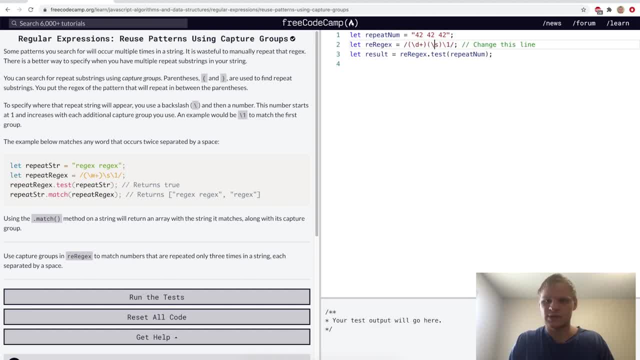 so i think i need to put parentheses and then backslash one, and then backslash one and then backslash s plus, and then i can do backslash one and backslash two and then backslash one. so i'll check if it's a digit and then it'll check if there's a space and then it'll check if there's. 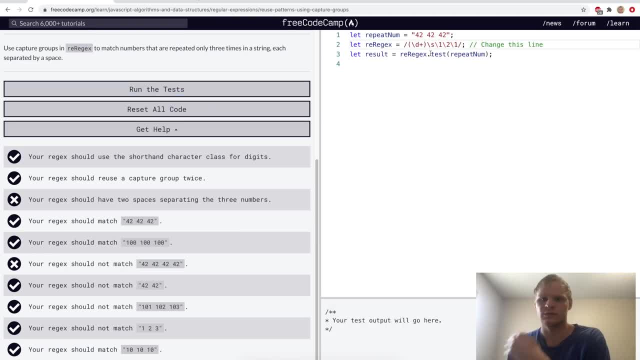 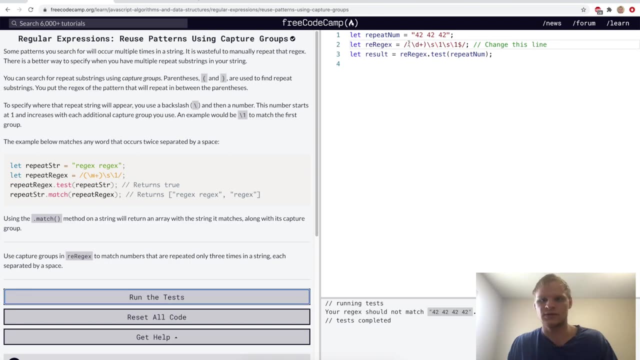 a digit again. let's try this out. no, okay, i guess it's no parentheses or backslash s and it'll just be backslash one, then another backslash s instead of backslash two, and then backslash one dollar sign to check at the end, and then i guess this works, so we'll run it. what so we have to check if 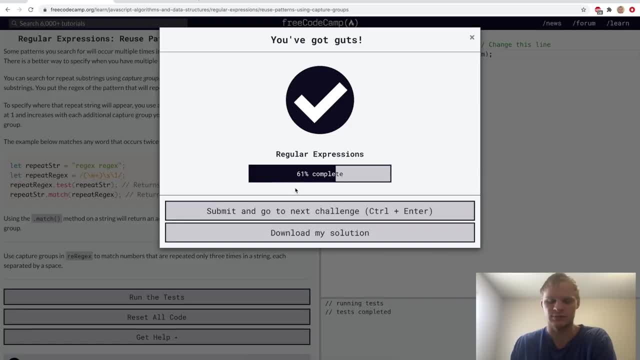 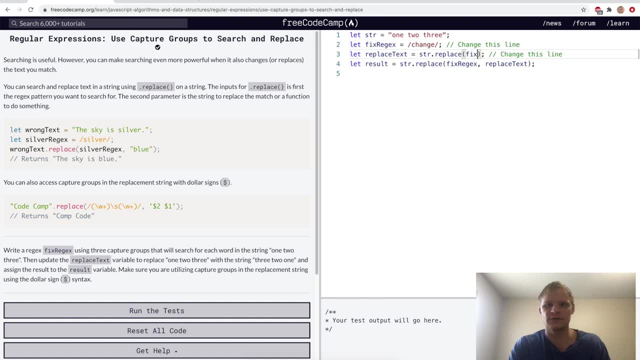 this is at the start, with the carrot, i guess, and then i'll go back to the first one, and then i'll it'll work, yep, okay, use capture groups to search and replace. so here we want to do string dot replace, and then we want to do our fixed rejects, and then we want 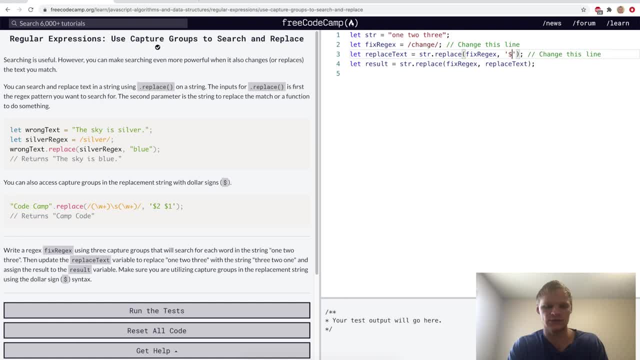 to do dollar sign three, dollar sign one. yeah, we'll go dollar sign three and dollar sign two, then dollar sign one, and then we'll grab the three words using our capture groups. so we'll go with parentheses- we need three parentheses- and we'll do spaces in between them and it'll be backslash word plus for all. 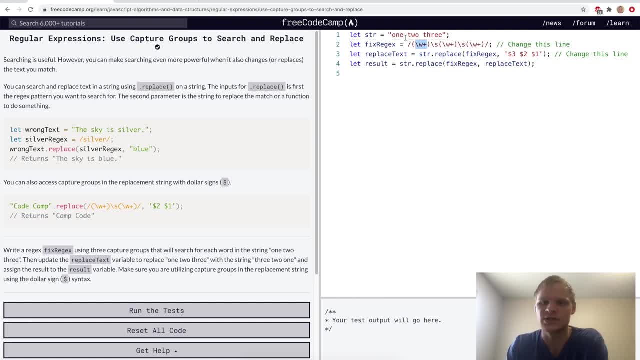 three of these, or backsplash character plus. so these will match up with one, two and three, and then there's spaces in between and then this will switch the order of them. so it'll take three and put it on to the first one and it'll take two. keep it where it is, it'll take one and move it to the end. actually, I 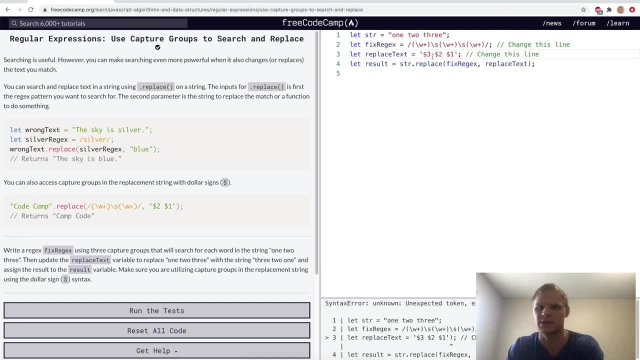 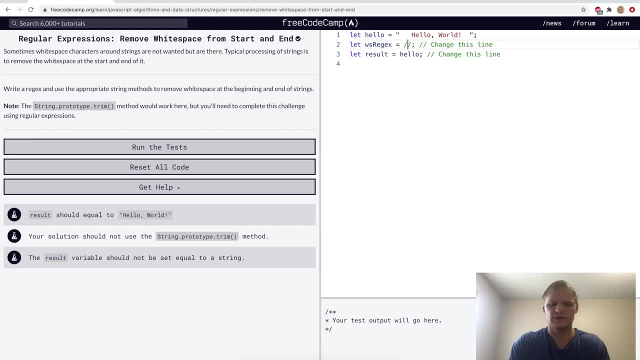 can get rid of this string dot replace, because they already do it for me, and instead just do dollar sign, three dollars and two dollars on one, and let's try that yep, remove white space from start and end. so I'm guessing here we can do caret and then do a grouping of